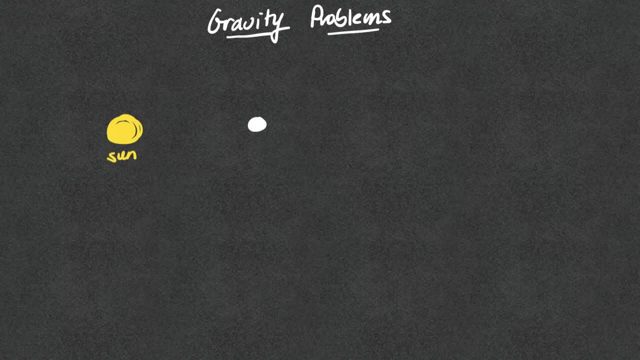 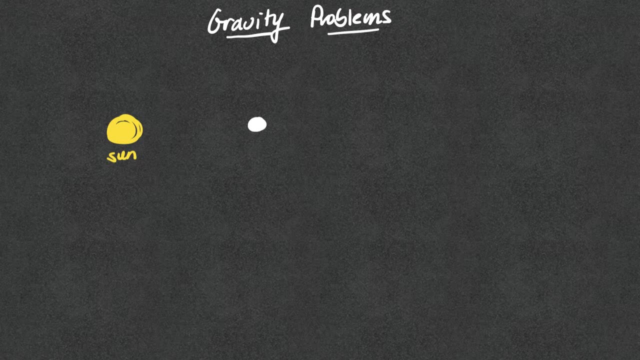 picture. Just keep that in mind. It's really hard to do a scale picture of the solar system for some really cool reasons that you learn if you take astronomy. But so here's the Earth, And then you know Mercury, Venus, Earth, Mars, And so here's Mars, which is a little further away. 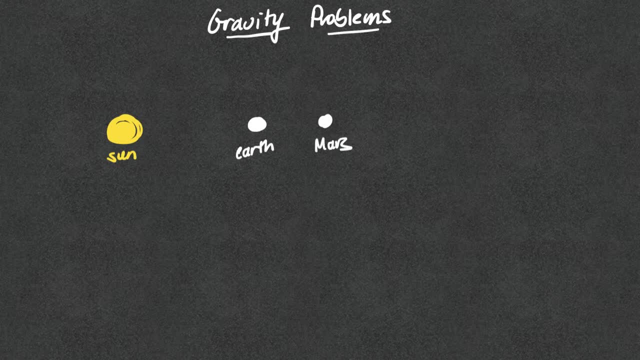 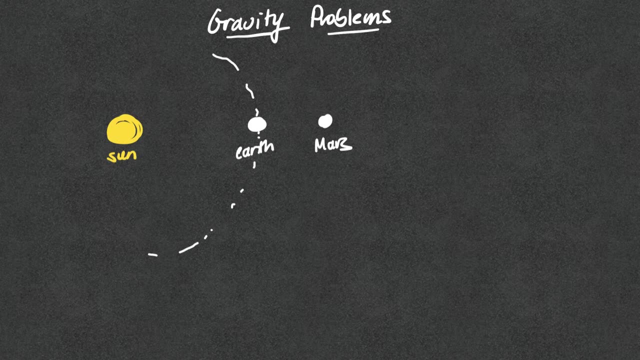 and a tiny bit smaller. And if we approximate, what's good about using Earth and Mars is planets don't really revolve around the sun in circular orbits. Mars and Earth have pretty like close to circular orbits. In fact, the orbit of Mars was so close to circular that Johannes Kepler actually 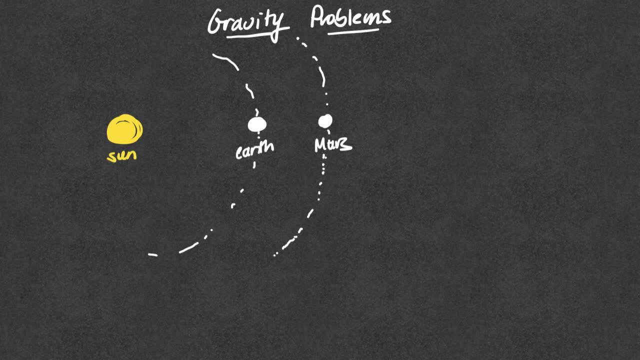 that, you know, people thought it was a circle for a long time And Kepler, it was the tiniest little amount off from a circle And he was able to figure that out- an astronomer named Kepler. Okay, so we have some distances. we have the radius of the Earth's orbit. I'll call it capital. 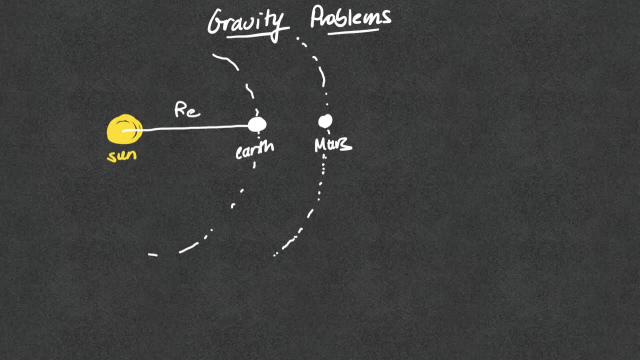 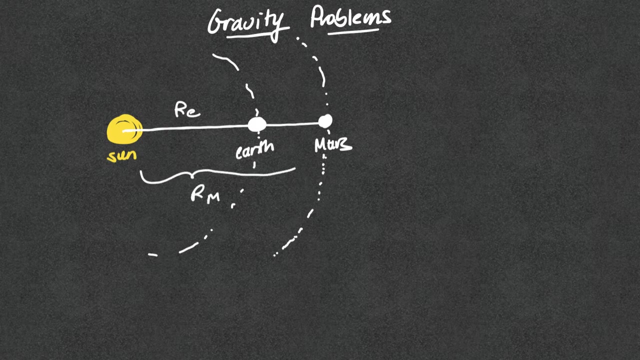 RE: Important not to confuse that with the actual radius of the Earth. you have to pay attention to whether you're looking at an orbital radius or a planetary radius. And then we also have the radius of Mars's orbit, which would be this whole distance And the radius of the Earth's orbit. 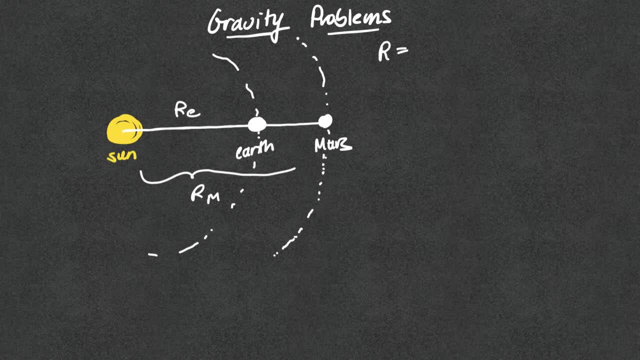 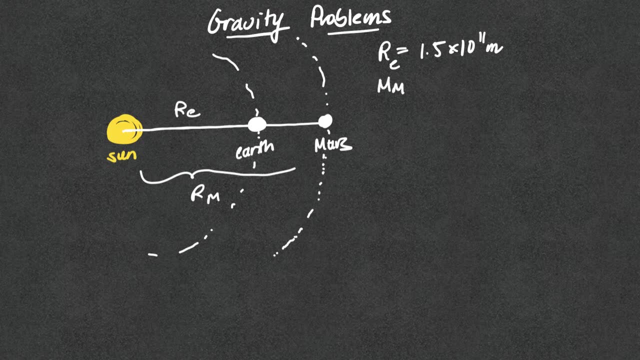 around the sun is 1.5 times 10 to the 11th meters. It's pretty far. And then the radius of Mars's orbit around the sun is a little further: it's 2.3 times 10 to the 11th meters, approximately. Okay, so what can we figure out? Well, we could. 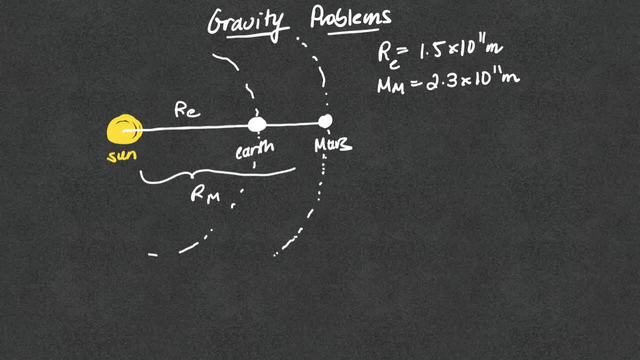 figure out the gravitational force between the Earth and the sun, the gravitational force between Mars and the sun. I want to actually figure out the gravitational force between the Earth and Mars when they're, you know, as close as they get, And so 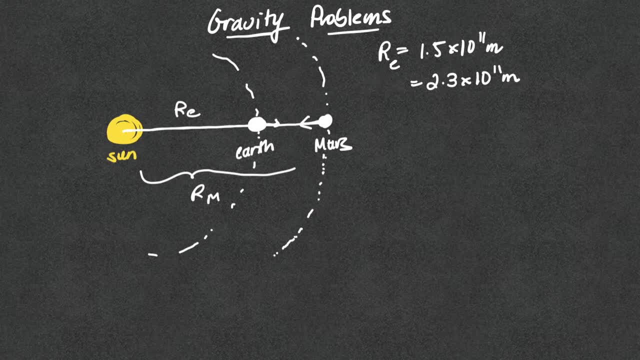 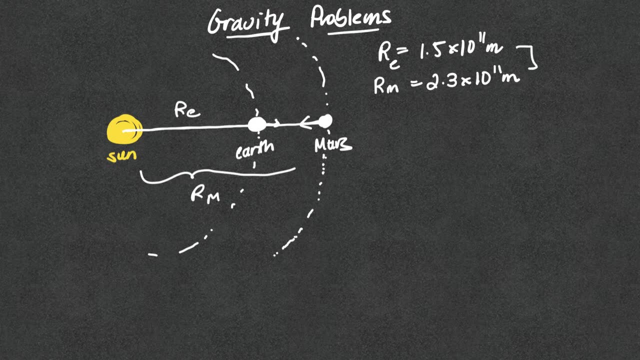 in order to do that. this is a radius, by the way: M radius of Mars. is that Okay? I'm going to need to subtract these two numbers to get the distance D between the Earth and Mars when they're lined up like this in conjunction. So that distance, I'm going to call it little r, Earth-Mars, the radius. 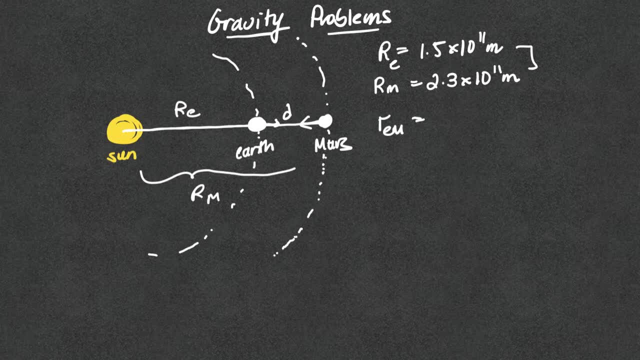 from Earth to Mars is going to be 1.5 times 10 to the 11th. sorry, 2.3 times 10 to the 11th, minus 1.5 times 10 to the 11th, And that, if you work it out, is 8 times 10 to the 10th meters. That's really far away. That's how far apart they are. 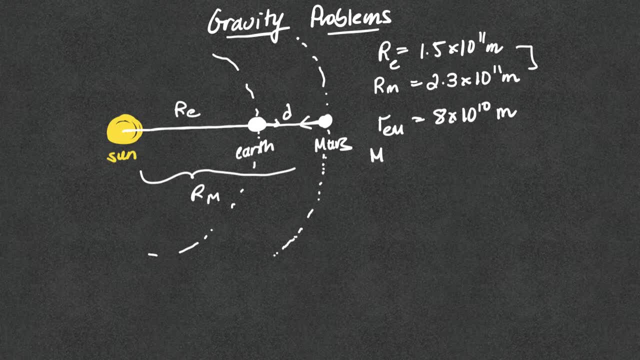 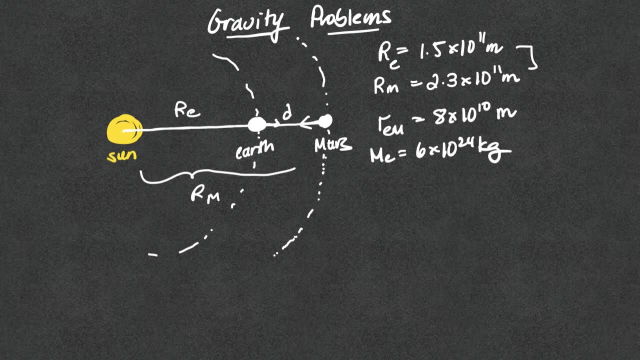 In order to do this calculation, I'm also going to need to know that the mass of the Earth is about 6 times 10 to the 24th kilograms, and I'm using round values here because this is more about the process than being super precise. 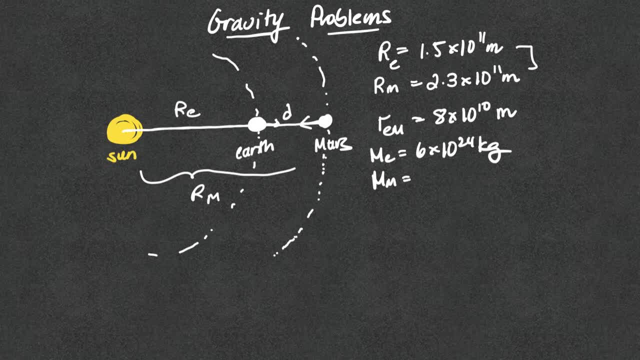 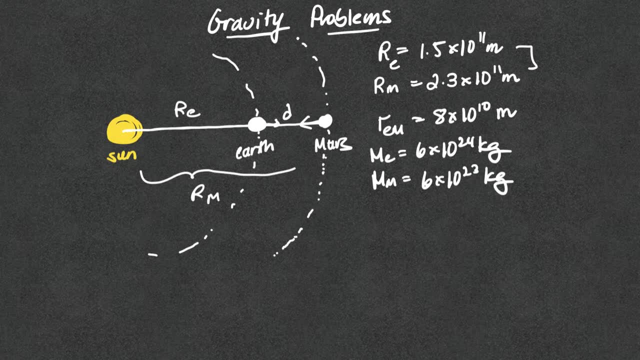 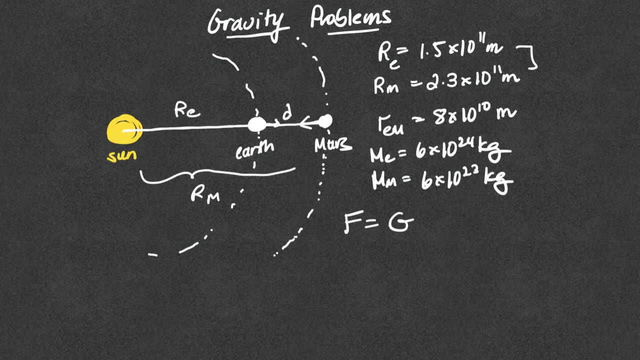 and the mass of Mars, which is about 10 times lighter, which is 6 times 10, to the 23 kilograms. Okay, so what's the force between them? That's where I use Newton's law of gravitation. The force between any two things is capital G, the universal gravitational constant. 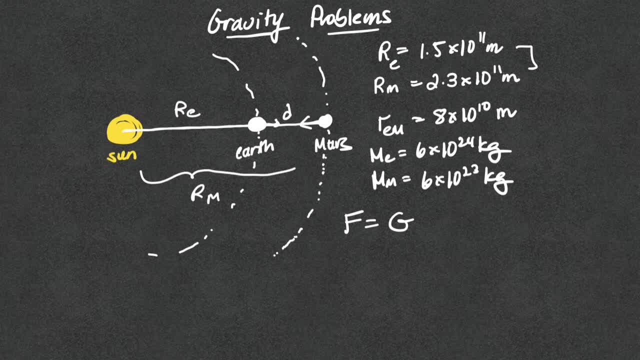 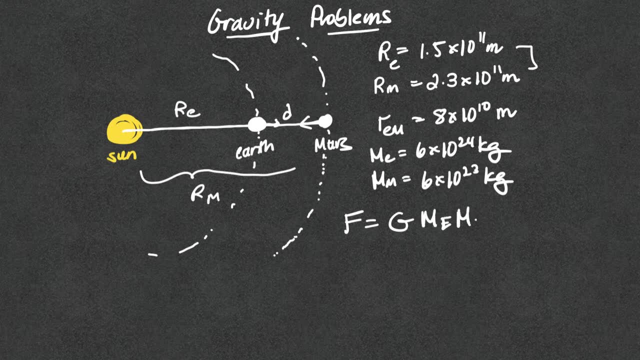 which is big G, but remember it's ironically really small. It's not little g- 9.8, it's big G. that cookie constant times the mass of the Earth, times the mass of Mars divided by the distance between them squared. So let's plug in some numbers and see what we get. 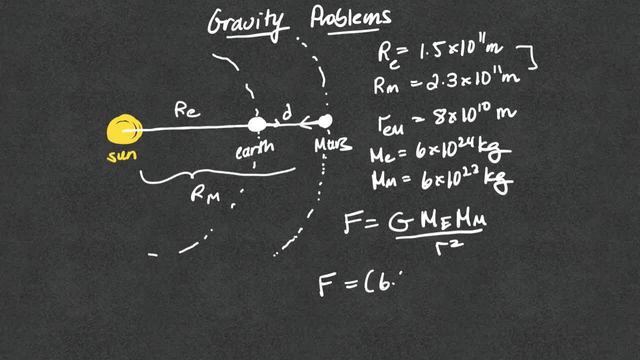 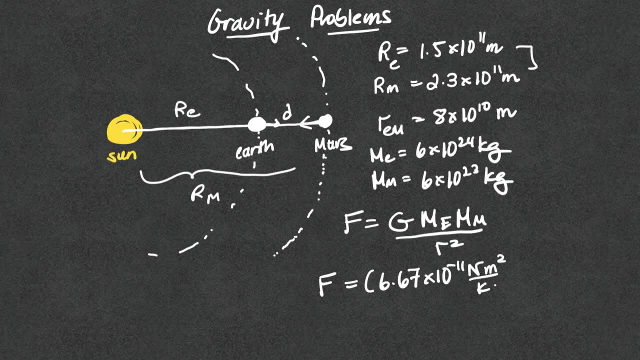 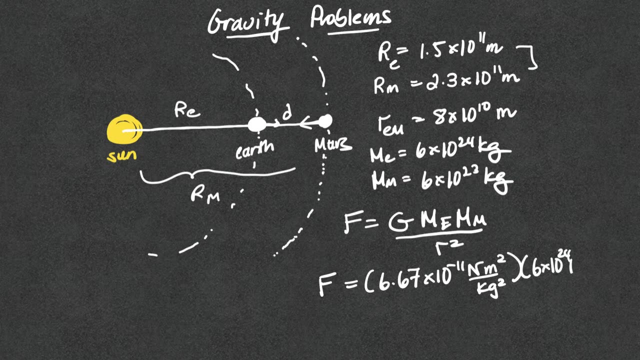 The force between the Earth and Mars is equal to G, which is 6.67 times 10 to the negative 11th. and it has those funky units, newtons meters squared per kilogram squared, and that's so that the force works out to newtons times, 6 times 10 to the 24th kilograms. 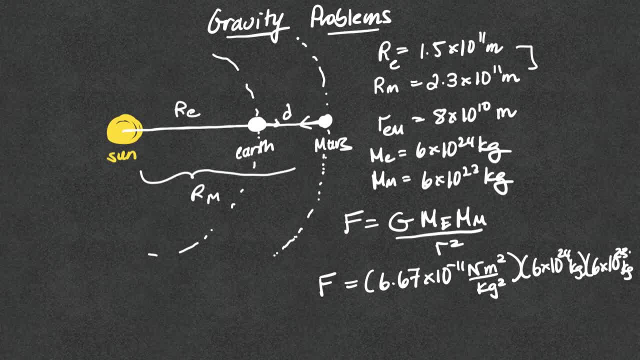 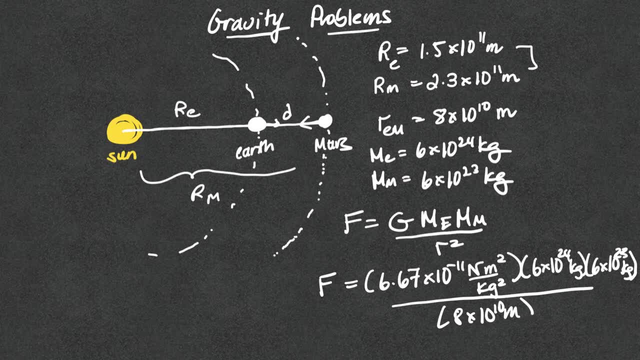 times 6 times 10 to the 23rd kilograms. I'm squeezing it in. divided by 8 times 10 to the 10th meters squared. Now possibly Pause and type this into your calculator. See what number you get for this force. 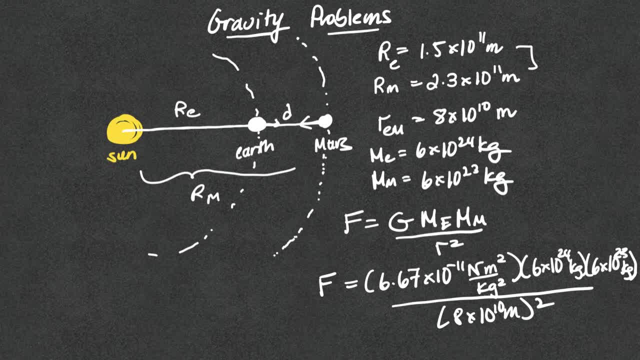 The way I do it is. I use for exponents the double E button on my calculator. It's better than using times 10 carat. You don't need as many parentheses. When I do squared, I do the squared button. I don't do carat 2.. There's a lot of little tricks. 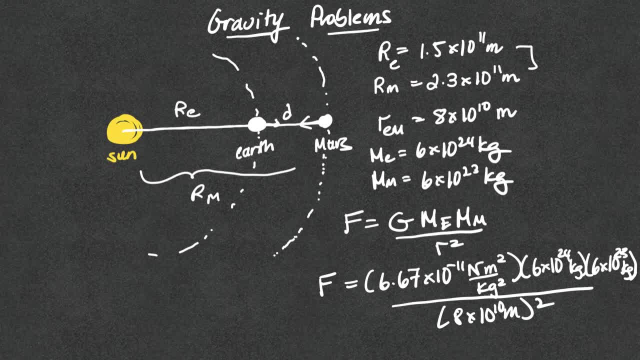 When we're in class together. we'll practice typing these in, I promise. But if you work it out, the number that you get for the force between the Earth and the Mars when they're at closest approach is Drumroll, 3.8 times 10 to the 16 newtons. 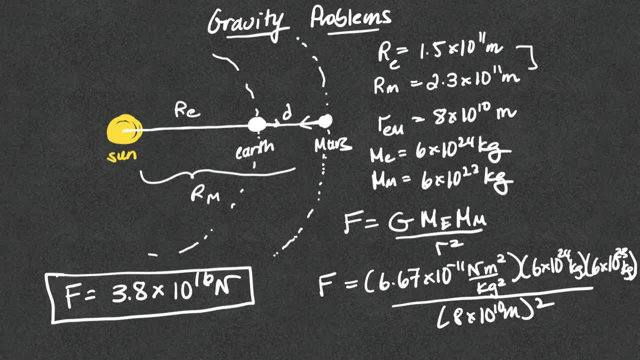 So that's how you calculate Now. you'll get an intuition for these values as you go. There's really no way to know if that's right. right, Like you don't know, but like, yeah, that makes sense or that seems about right. 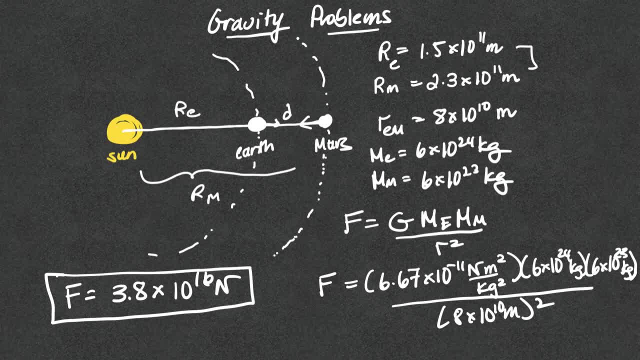 You can't really judge these forces, That's okay. It's really important to double check your calculations. Make sure you get the answer. You can get it twice. then you can be confident of the numbers you put in, that you know you didn't make a mistake. 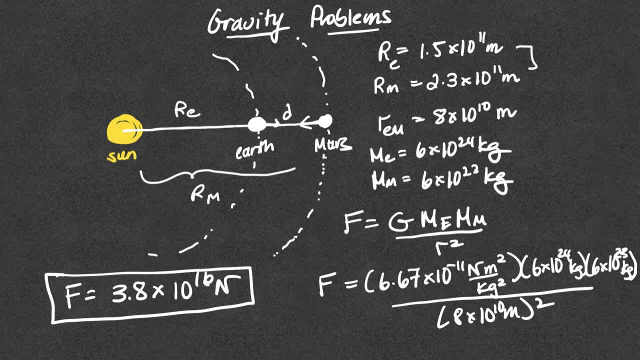 All right, All right. The next thing I want to calculate is: I want to use the law of orbits to calculate how long a Martian year is. How long does it take Mars to orbit around the Sun? So that's my next thing. I'm going to go to the next page. 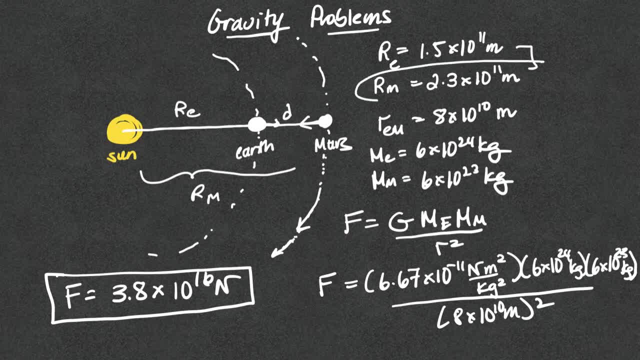 I want you to keep this picture in mind. We're going to need the radius of Mars's orbit for that- 2.3 times 10 to the 11th meters, And we're going to need the mass of the Sun, which I'll have on the next page. 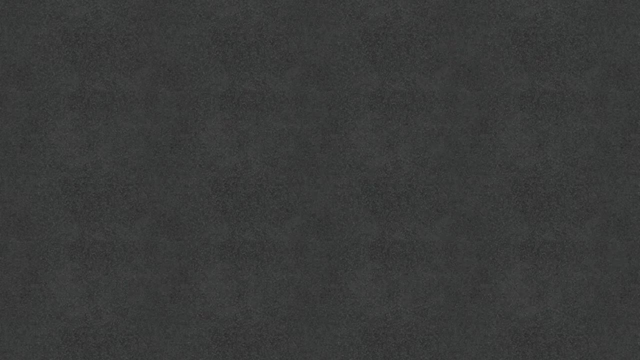 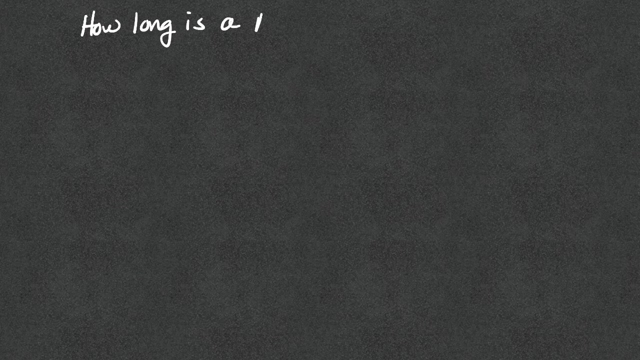 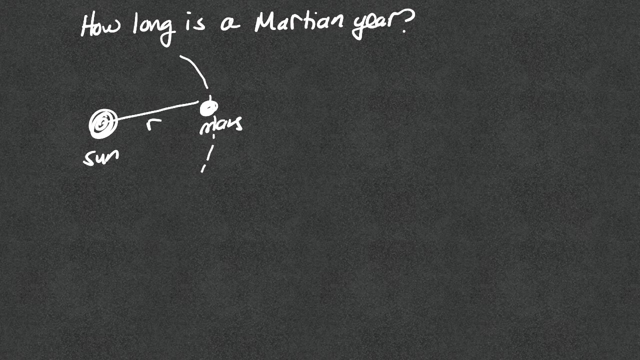 So we want to know: how long does it take Mars to go around the Sun? Okay, How long is a Martian year? Okay, so we have the same picture. We have the Sun, We have Mars. Mars is orbiting the Sun at a distance r. 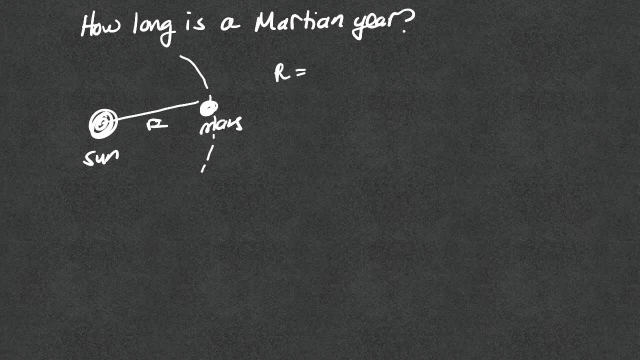 And that radius r is equal to what did I say, 2.3 times 10 to the 11th meters. Now remember, in the law of orbit, the radius of Mars is equal to what did I say: 2.3 times 10 to the 11th meters. 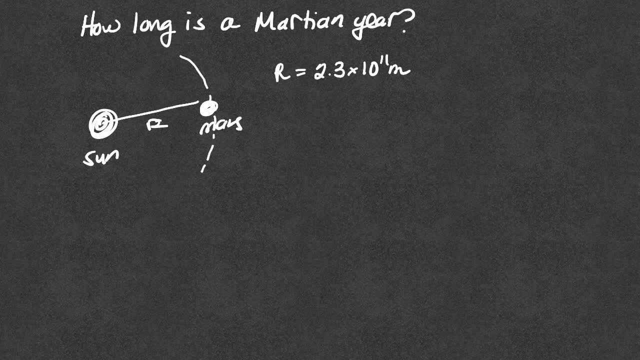 Now remember, in the law of orbit, the radius of Mars is equal to what did I say? 2.3 times 10 to the 11th meters. Now remember, in the law of orbits, the mass of the thing doing the orbiting drops out of the equation. 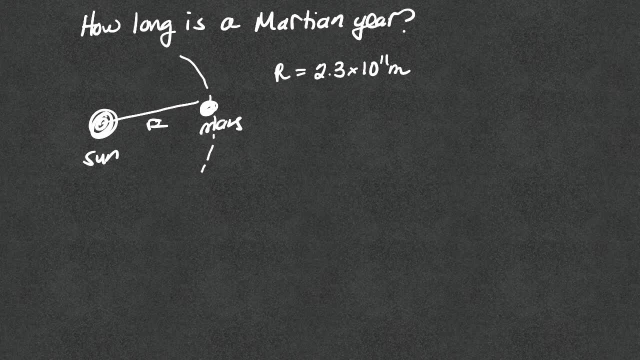 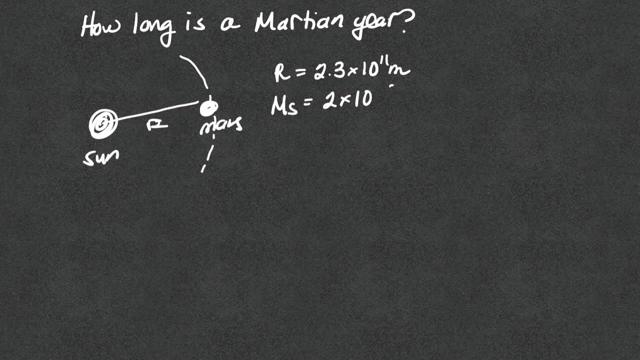 All that matters is the mass of the thing at the middle. So here we're going to need the mass of the Sun, which is approximately 2 times 10 to the. that is not right. I don't know why I'm writing different numbers than I say. 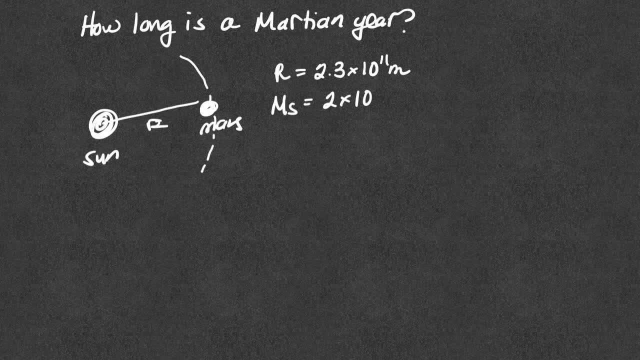 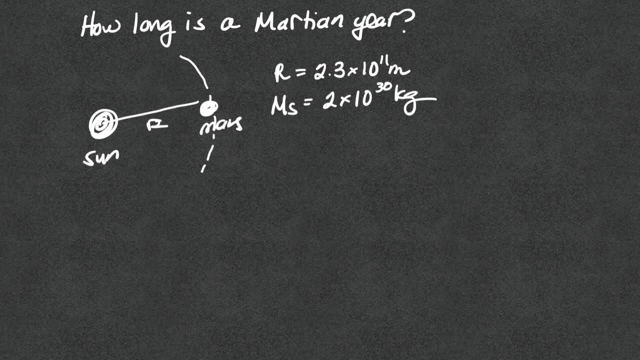 I had a trigonometry teacher who said one thing and wrote a completely different thing on the board, And it was really strange. She did that all the time. 2 times 10 to the 30 kilograms. Okay, Now remember the law of orbits which we derived. 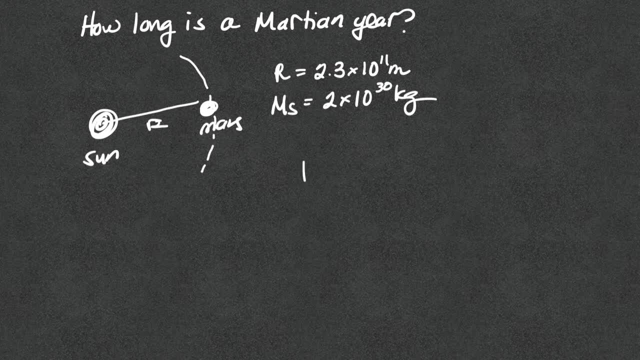 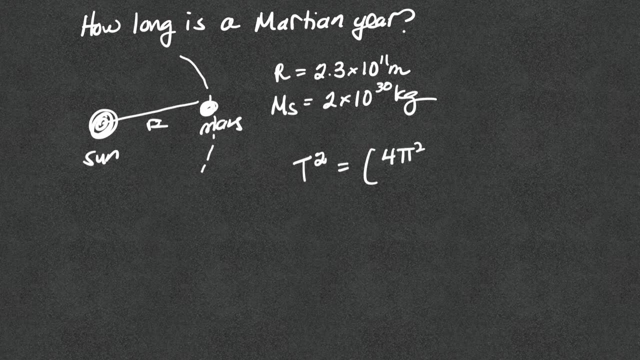 which you derived using circular motion, which is that t squared the period of orbit in seconds- very important- we're going to have to convert- is equal to 4 pi squared over g times the mass of the sun or the mass of the thing at the center. I'm just going to leave it as capital M. 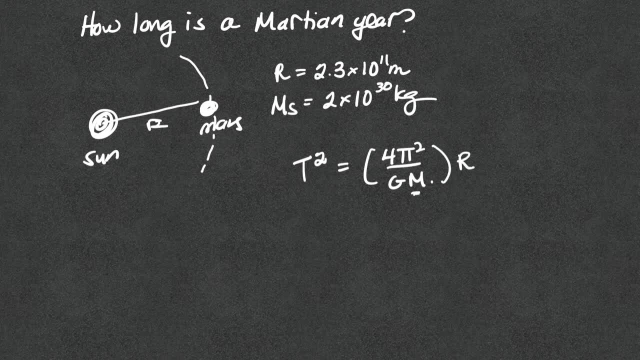 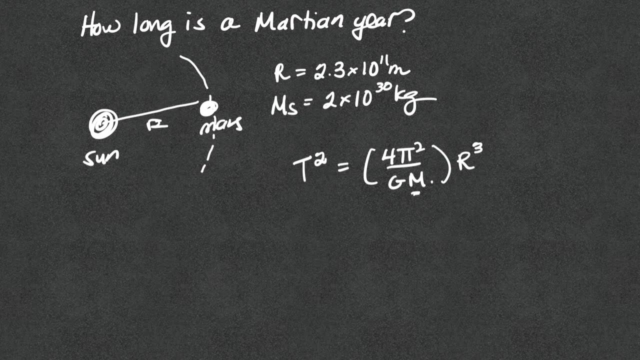 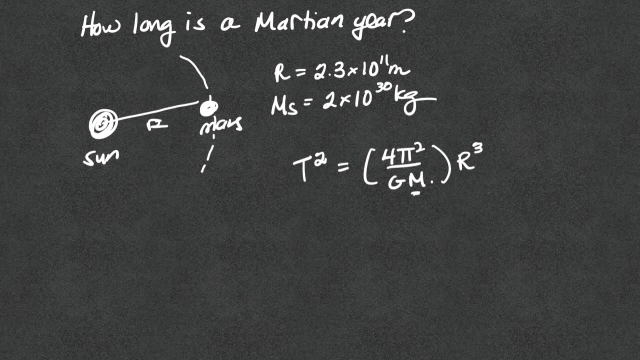 but that's the mass of the thing being orbited times the radius of the thing doing the orbit cubed, Not the radius of the planet, the radius of that planet's orbit. This is all about orbits. Okay, a couple of you asked me like: why is the r outside the parentheses? Can't it just be in the? 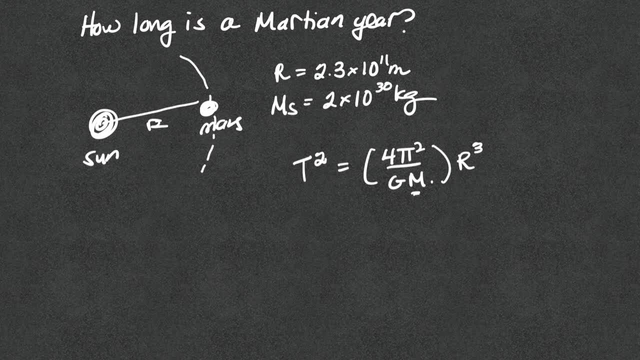 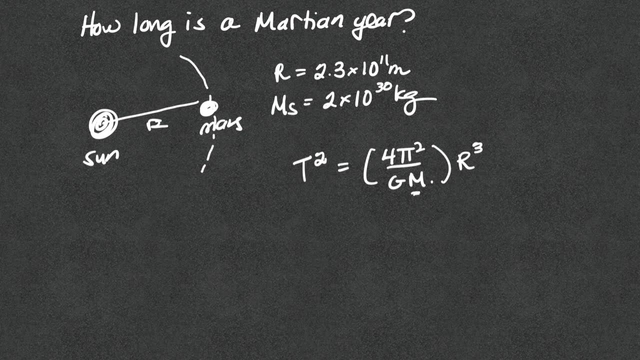 numerator? It can. Those are mathematically equivalent, remember, because you're just multiplying a straight line. but this can be. you know, this is the way it's normally written. Let's solve for the period. So t squared equals 4 pi squared. that's just numbers. 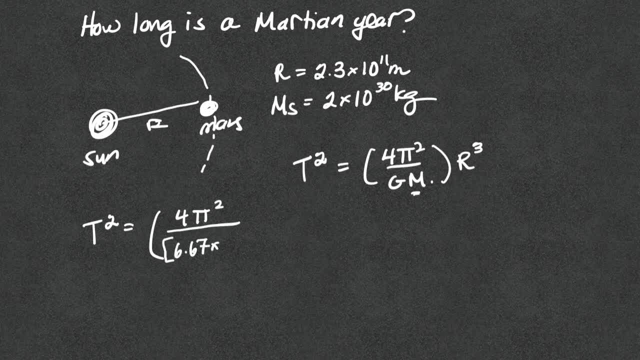 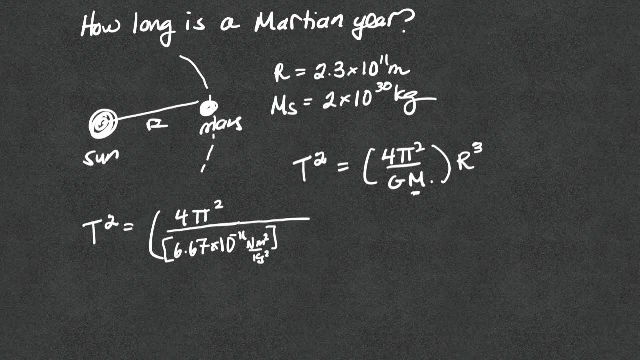 divided by g, which is 6.67 times 10 to the minus 11, squeeze this in newton meters squared per kilogram, squared divided by the mass of the sun, which is 2 times 10 to the 30 kilograms. 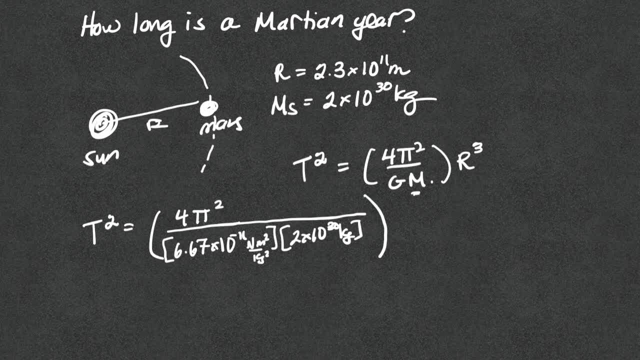 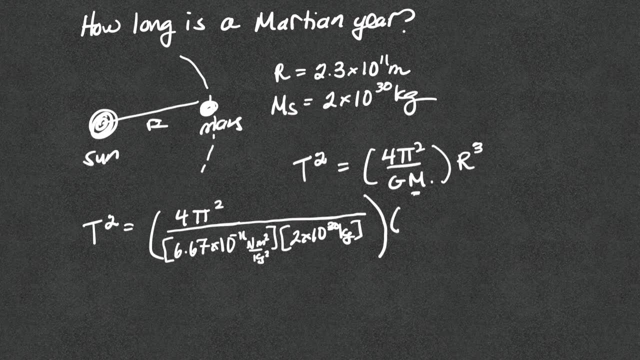 You might be like: where's that kilograms going to go? How does this work out? Remember newtons. you can break down into more fundamental units. The units will always work out every time. Let's put the orbital radius in now, 2.3 times 10, to the 11th meters. and don't forget to. 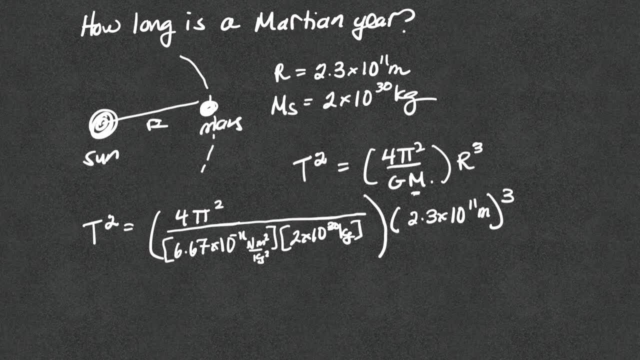 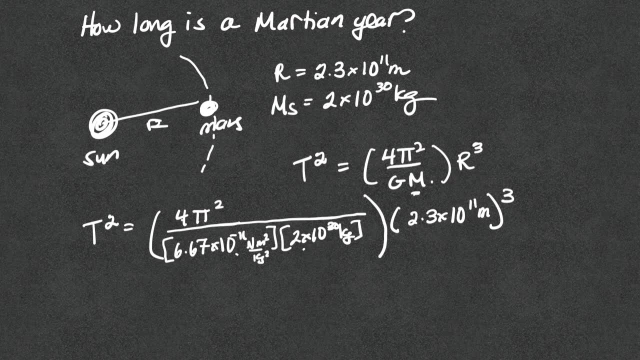 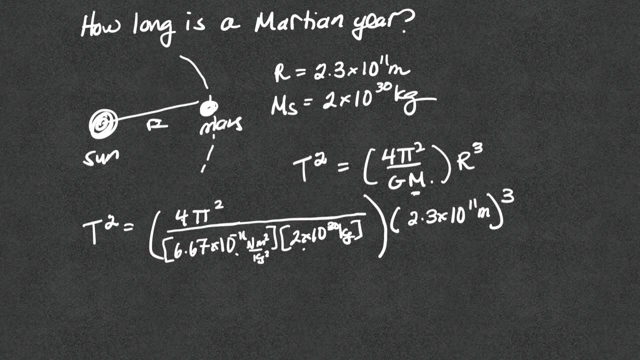 cube it. So the way I would do this is, I think I would first multiply these two things in the basement, then I would invert that, then I would multiply by 4, then by pi squared and then by 2.3 times 10 to the 11th cubed. That's how I would go about this. If I did that, I would get that. 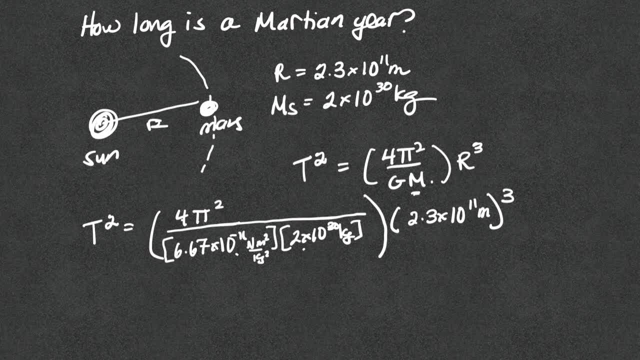 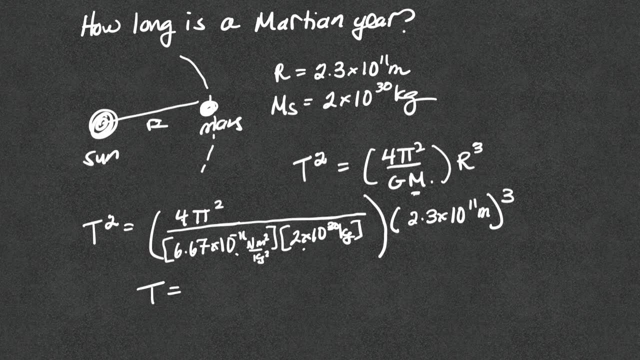 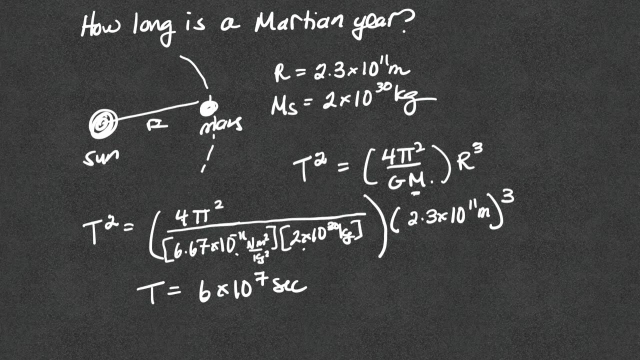 t squared is some big number and then I would take the square root. If you do the square root, pause it. do the calculations out and see if you get this. I get about 6 times times 10 to the 7th seconds. A good rule of thumb is that an Earth year is about pi times 10 to the